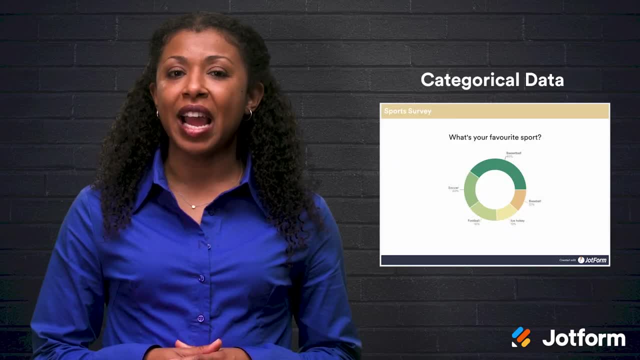 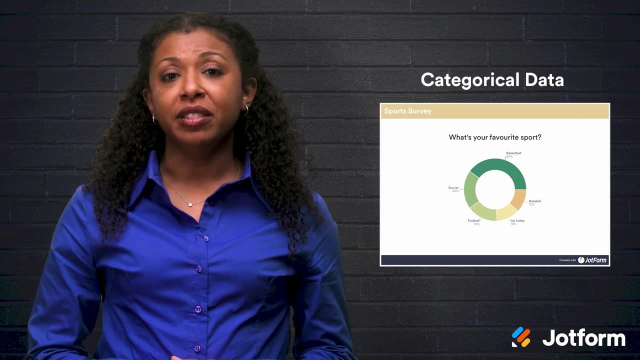 Let's start with categorical. When a customer gets to choose an answer from a predetermined list of responses, this is known as categorical. An example might be the question: what is your favorite product feature? And they might have to choose between ease of use. 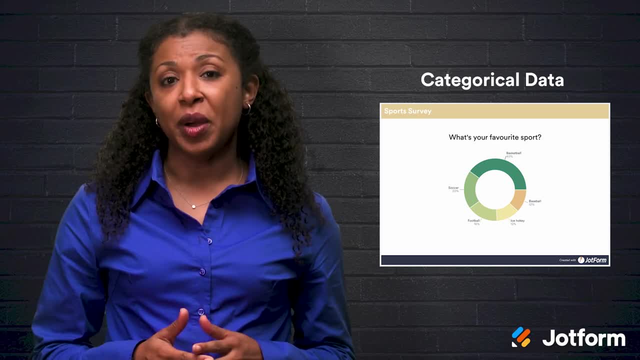 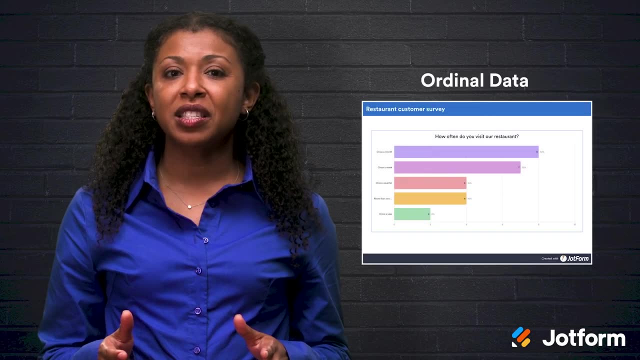 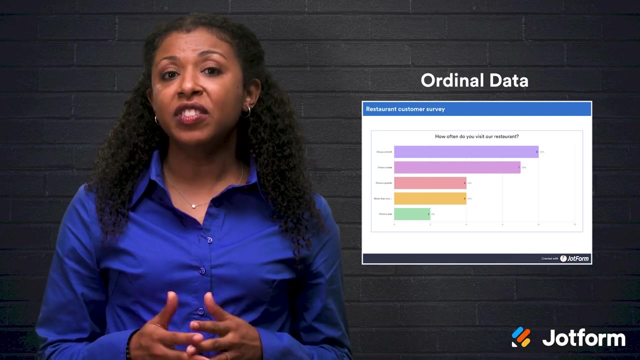 size and affordability. These are simple to evaluate. It involves counting and dividing the information to see the most popular responses. If the customer's responses fall into a logical order, then you are gathering ordinal data. An example might be the question: how often do you visit our restaurant? 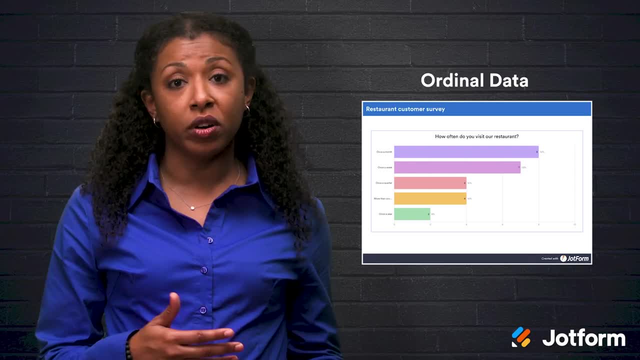 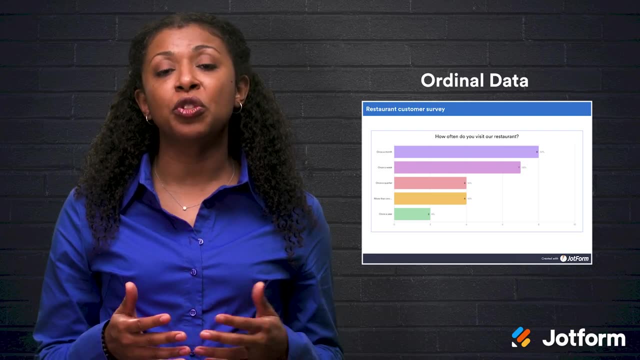 Potential answers could be rarely: once a year, once a quarter, weekly, et cetera. The purpose of this type of question is to see how often your customers are interacting with your product or service. For the next set of questions, we're going to be asking questions that are asking. 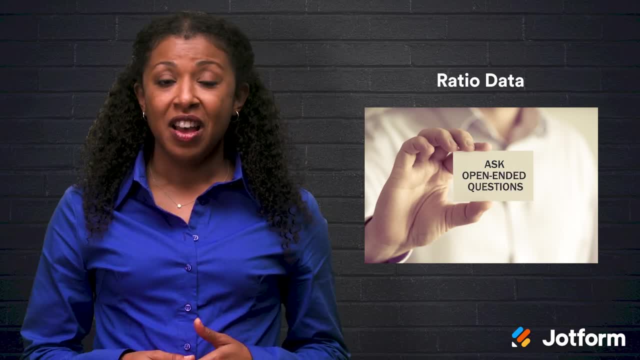 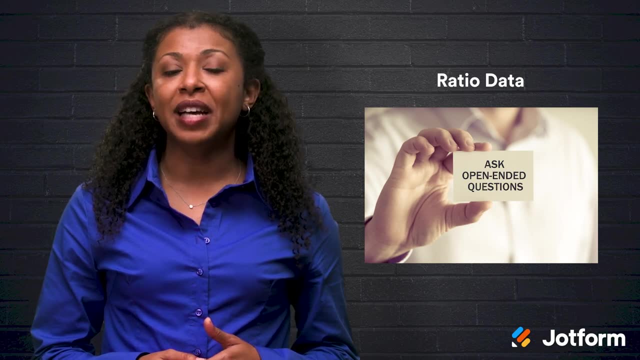 for precise information, that is, ratio data, For example, you might talk about a customer's budget- providing an open-ended answer field. This data can be helpful in looking at measures of variance, of calculating averages- The last question type we're going to look at. 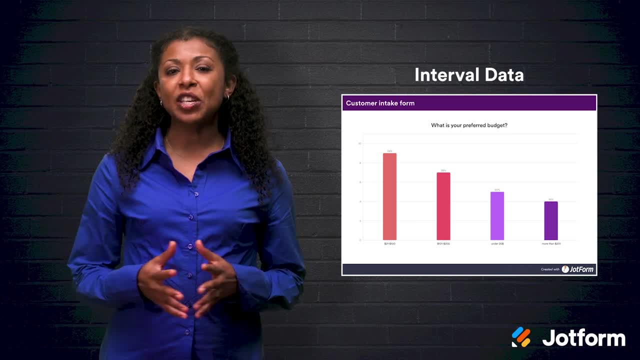 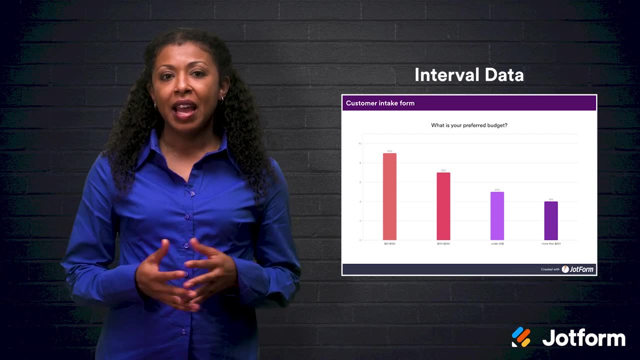 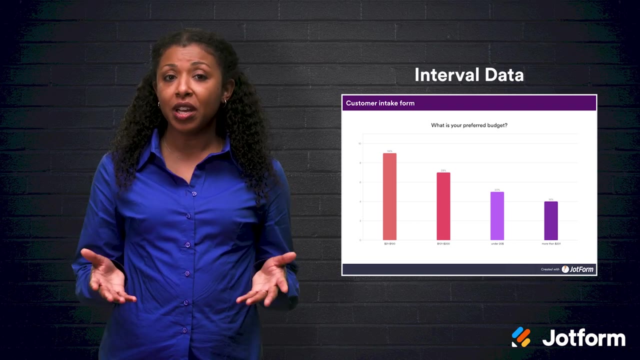 is interval data. This is a great way of segmenting your customers, so each group gets the right set of questions. An example is asking about their preferred budget and giving them potential answers listing predetermined amounts such as less than $20,, 21 to $100, 101 to $200, et cetera. 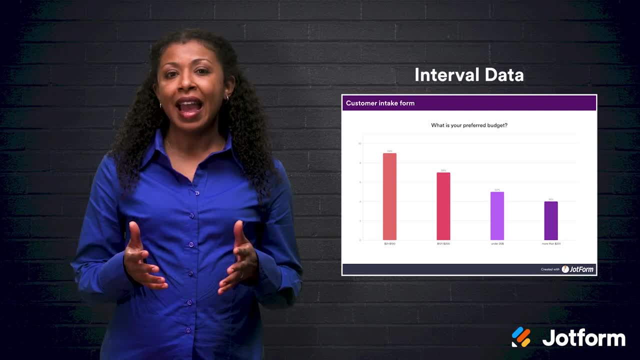 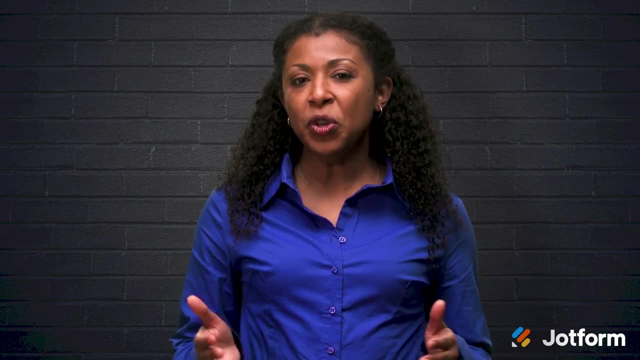 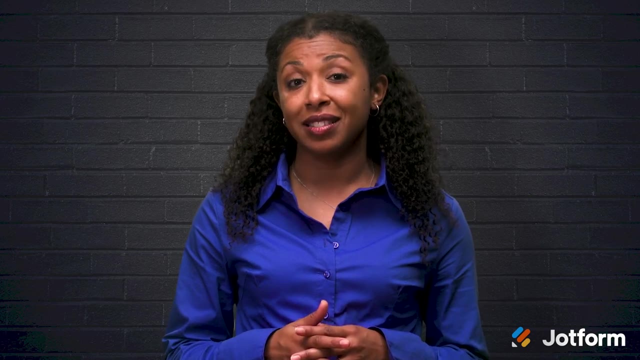 These are especially helpful when intervals are equally sized and you can calculate data averages. That brings up an important question: Do you need to go in a certain order when reviewing these questions? Crunching the number of questions first gives you a foundation to use when looking at the open-ended responses. 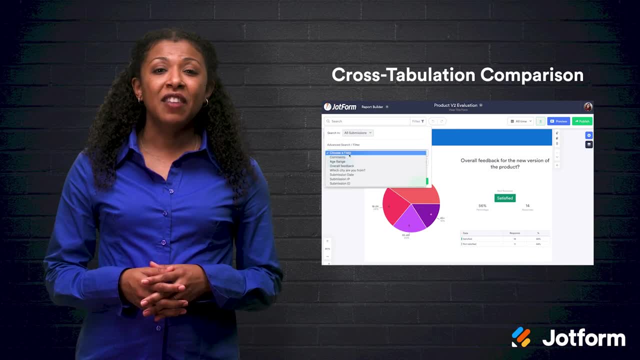 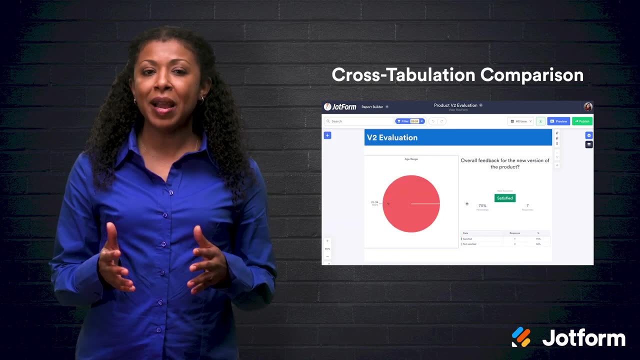 Now that we know our question types, let's move on. If you want to gain more insight from survey results, it will be helpful to use cross-tabulation in your analysis. This process basically puts the data into context so you can see the factors. 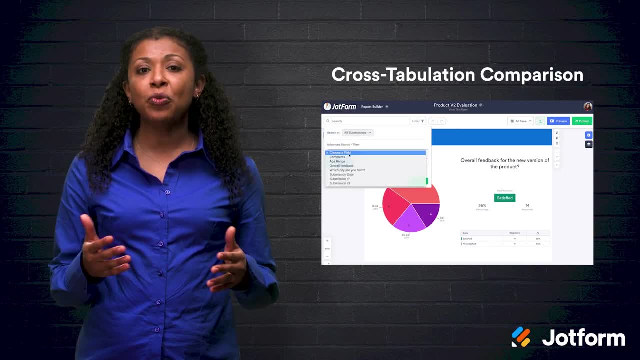 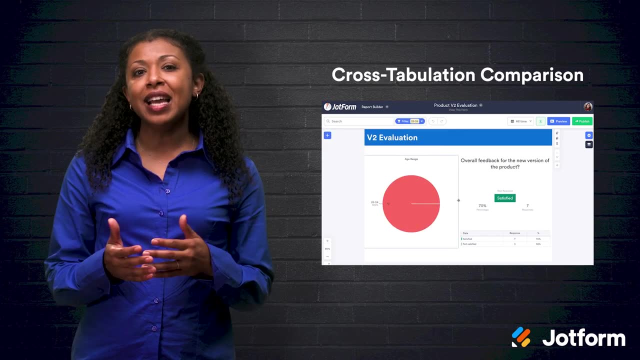 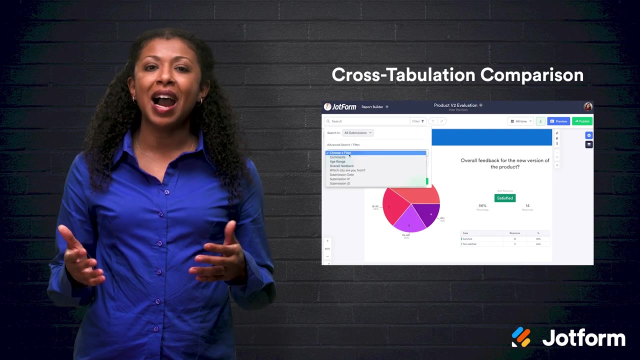 that might affect specific outcomes. It's also a great way to see how different groups of people respond to the same questions. With cross-tabulation, you can see how different age groups or other categories might have answered differently. For example, let's say that 56% were highly satisfied. 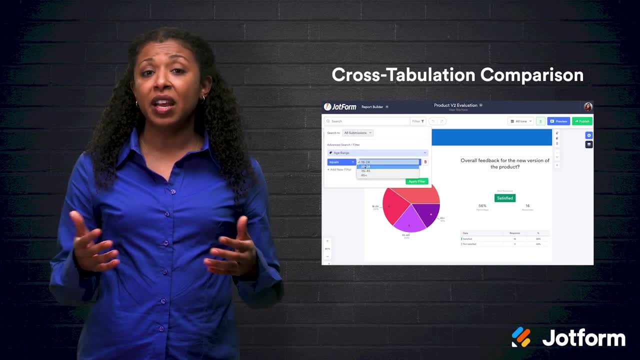 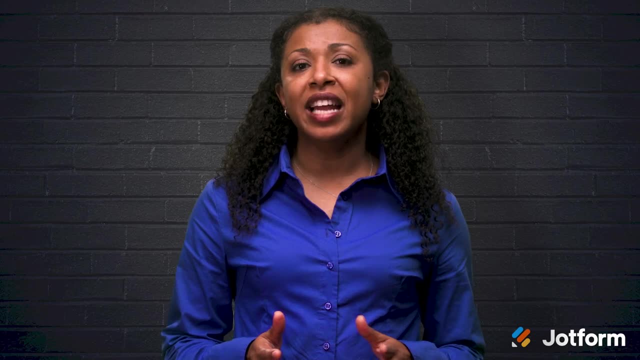 and 44% were dissatisfied. Is there something else we can identify to see who answered that? Can we break that down any further? You might find that the satisfaction levels change with age, budget or other reasons relevant to your target demographic. 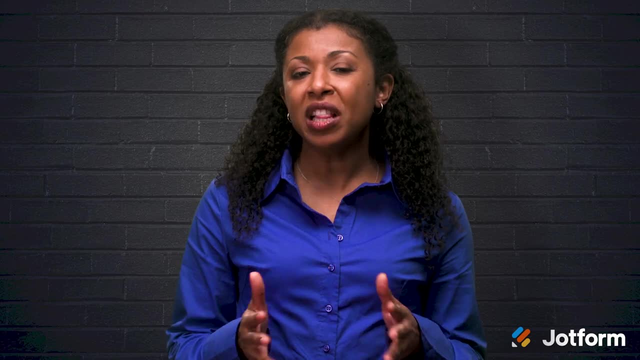 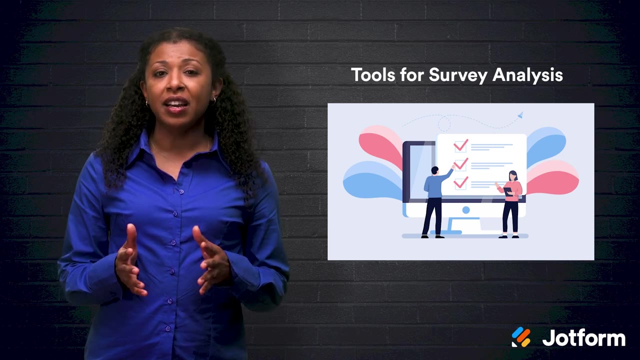 Through cross-tabulation, you might find some interesting, relevant data to use in your business. What if you need help with analyzing your survey results? If you're surveying a large number of participants every few months, it might be helpful to use a survey tool. 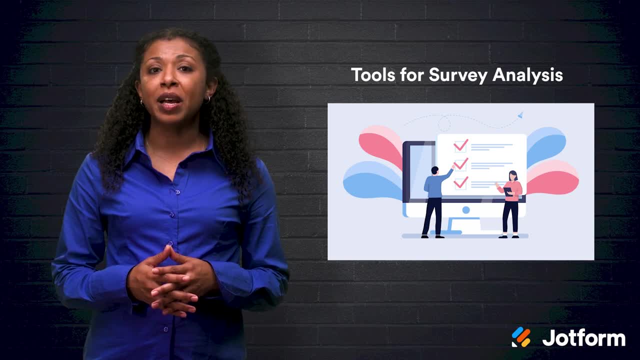 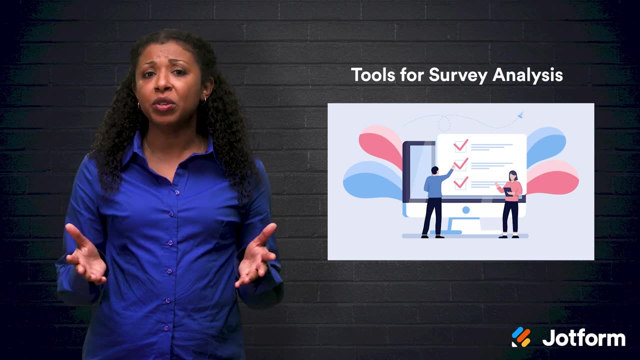 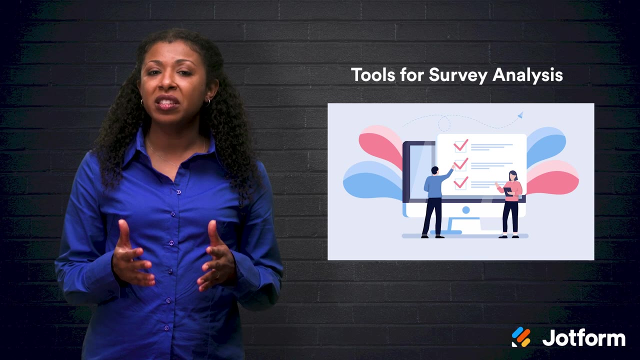 to analyze the responses. Manual analysis works best when there are fewer than 100 responses, But who has the time to do it manually when you need to evaluate hundreds or thousands of survey responses? When you consider the time requirements of manual analysis, it might end up costing you more. 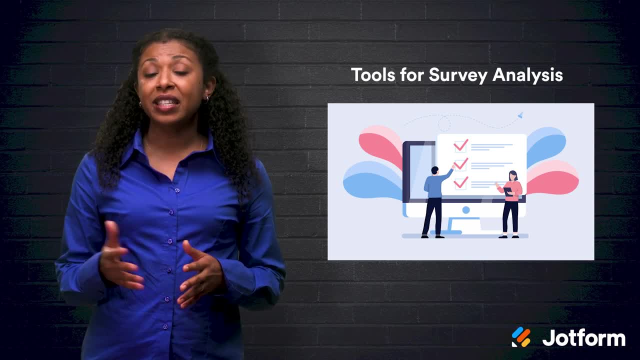 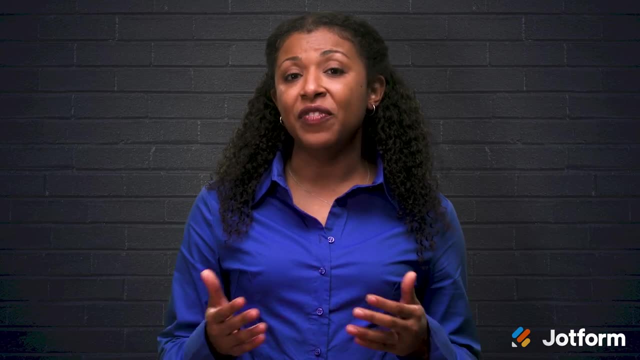 It also increases the likelihood of human error. Using Excel only works well if you know how to use the program's more technical features. When you're analyzing survey data effectively, you need to start at the beginning. Ask yourself: how am I gathering the information? 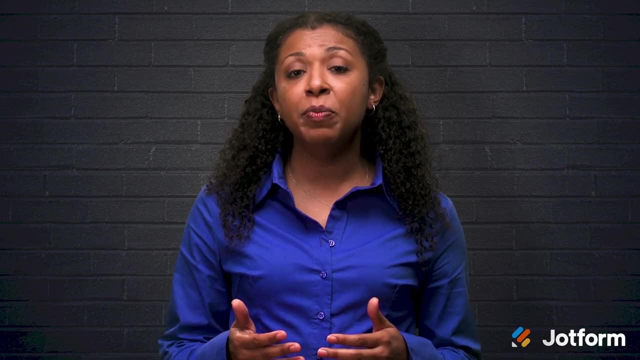 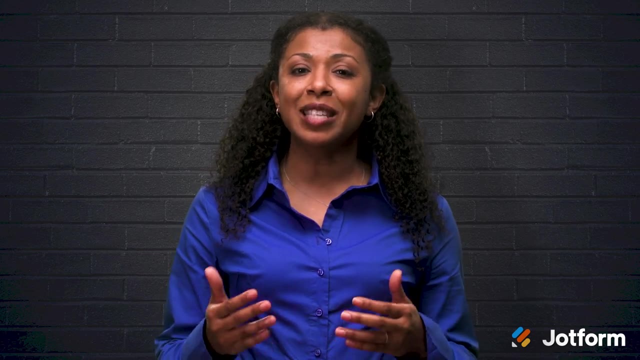 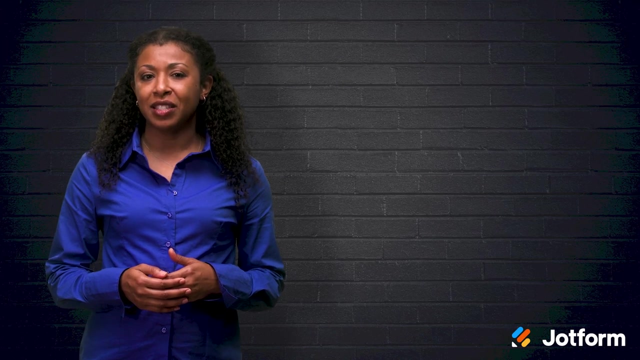 Efficient survey analysis tools include software programs with built-in features to consolidate data and compare results. JotForm has an online survey form that provides a simple answer to sharing a survey and collecting responses instantly. Let's look deeper at what JotForm has to offer. 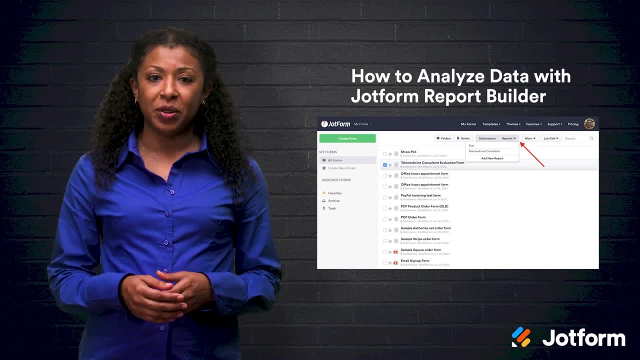 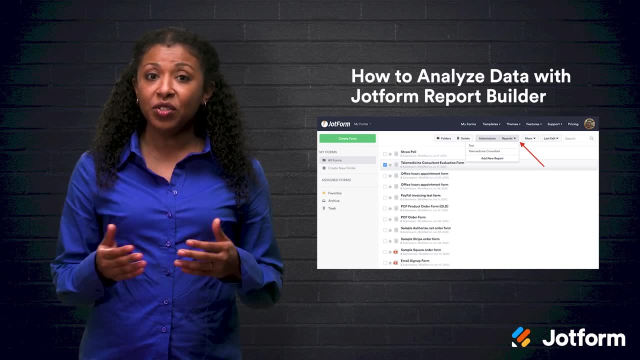 We're going to spend the rest of our time looking at the data, looking at JotForm's Report Builder. It can seamlessly transform data into charts and graphs that make data easy to understand. All you have to do is create an online form, share it. 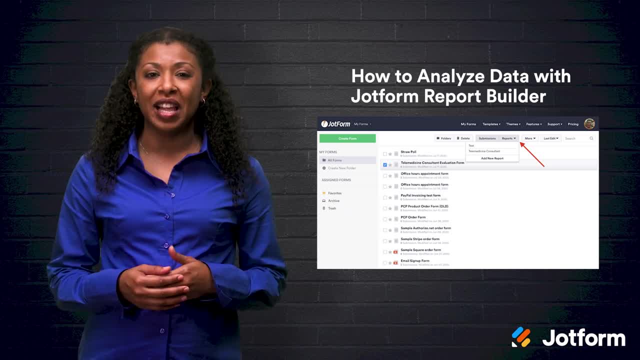 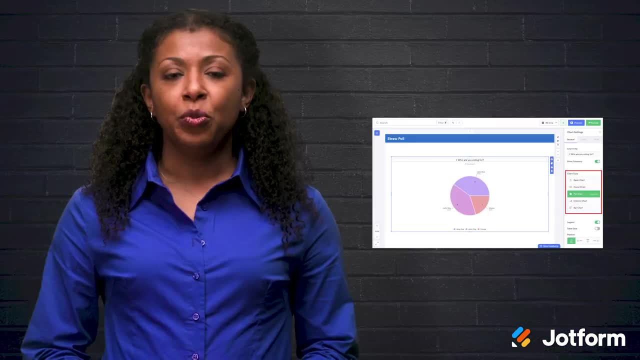 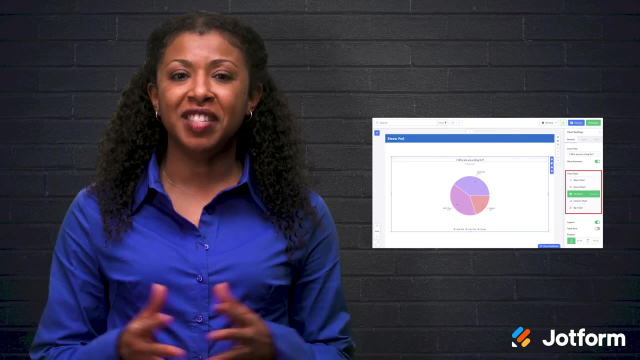 and use the Report Builder to create a presentation of the data you collected. Then you can automatically generate a professional-looking report or start with a blank slate. Regardless of whether you choose the built-in report or start from scratch, JotForm Report Builder offers a wide range of design options. 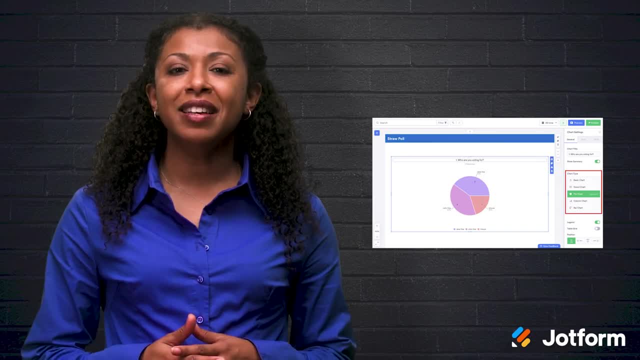 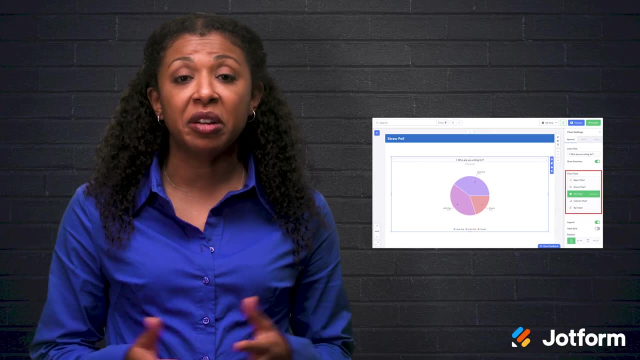 Which let you personalize your report and display the data the way you want to. If you want, you can add a business logo, upload a background photo, change fonts, et cetera. Along with changing the types of charts and graphs you have in your report, you can also show: 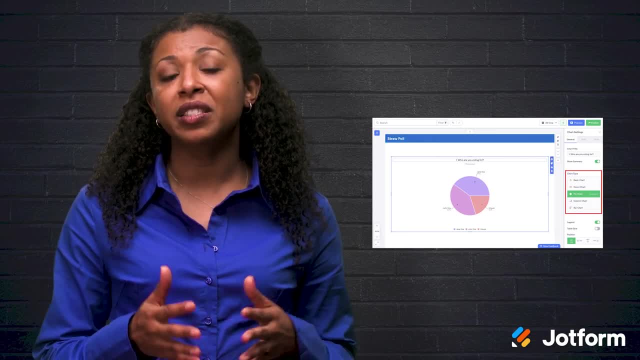 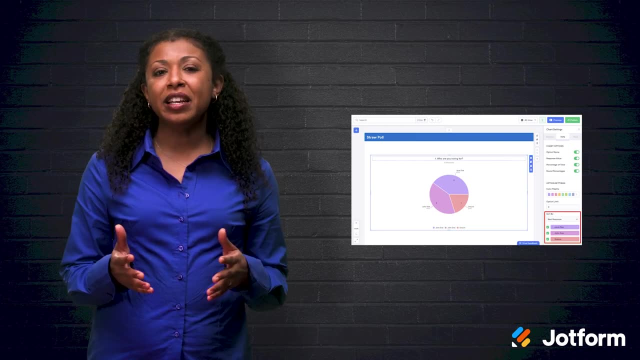 how many people answered a question, how many people selected a particular answer and how selected answers represent a certain percentage of all responses. You can make your data more understandable by rearranging the order or adding more data. For example, you can create a report. 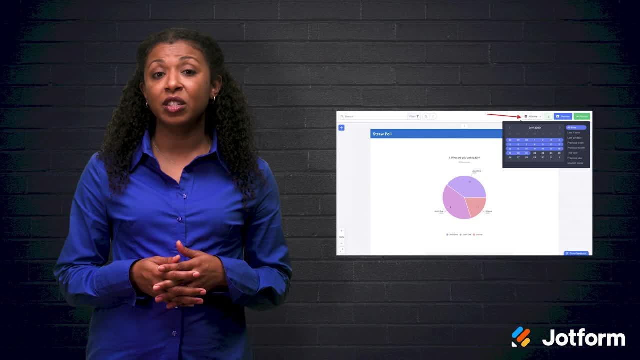 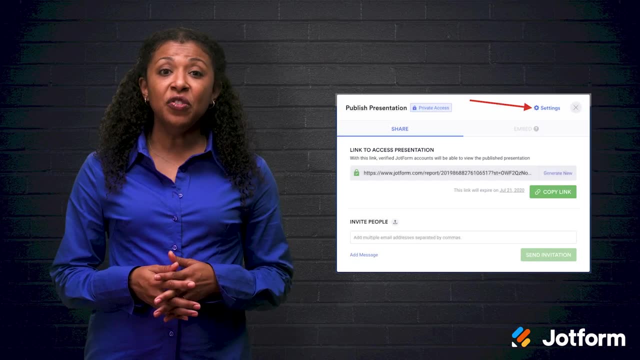 using a legend or table grid. JotForm Report Builder has the ability to analyze responses submitted within a certain timeframe or filter the data in your report based on answers to certain questions. After you've created your professional-looking report, you can download the report as a PDF. 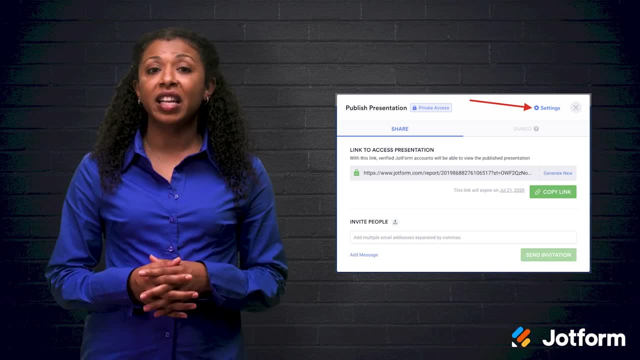 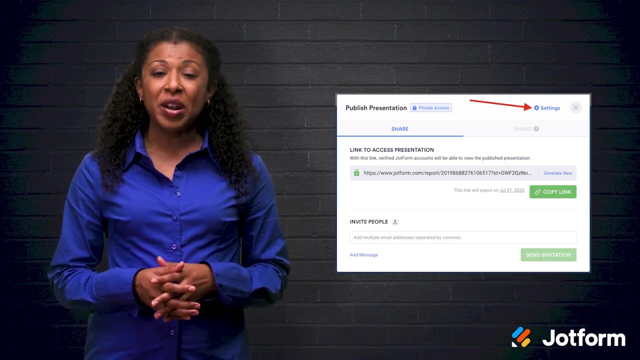 email it, print or embed it in a website. There are built-in safeguards that allow you to control who can see your report, determine how long they can access it and what they can do with it If someone fills out the online form. 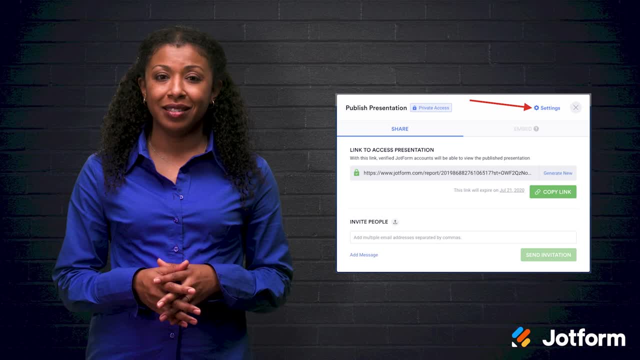 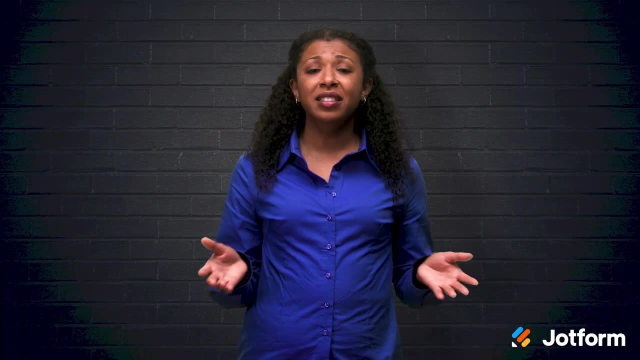 that is tied to a report, the information is automatically updated. No more wasting time manually recreating a report each time a new response comes in. When all is said and done, JotForm really is an all-in-one solution that lets you gather data and present it. 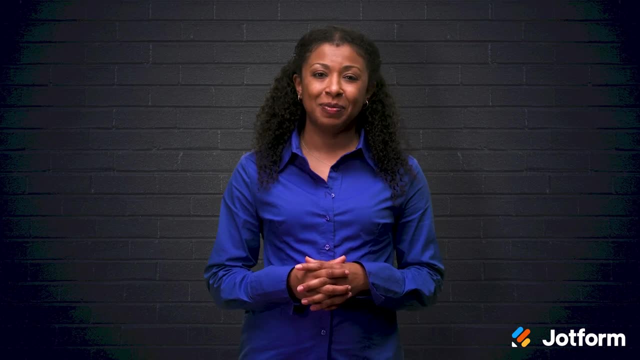 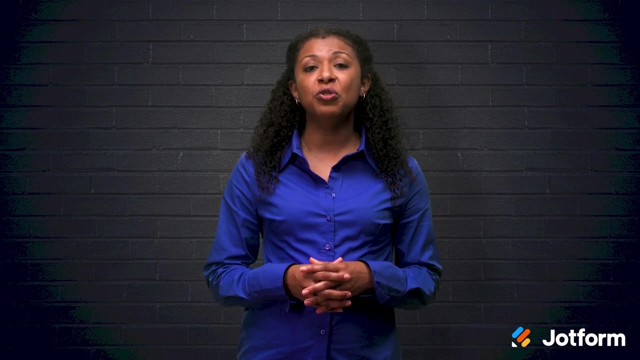 in creative, professional-looking reports in a matter of minutes, With features that display only relevant data, making it easier to understand. JotForm Report Builder can show you insights into your business and customers you might have missed before. It helps you make informed decisions. 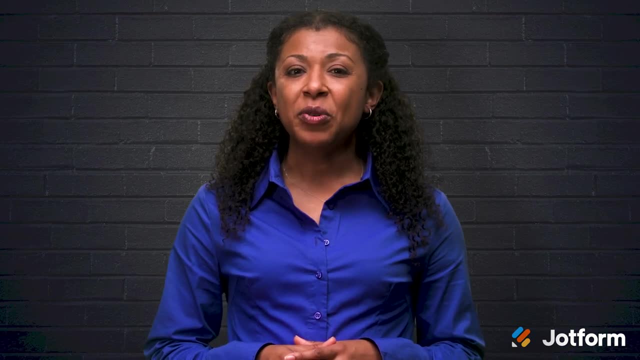 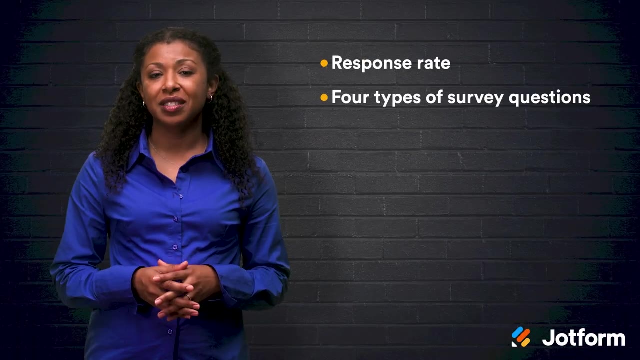 and come up with creative ideas. In today's video, we took a look at the following things when it comes to analyzing survey data Response rate. Four types of survey questions: Categorical data, Ordinal data, Ratio data, Interval data. 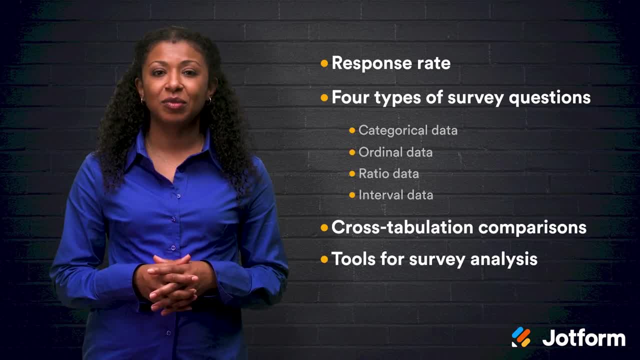 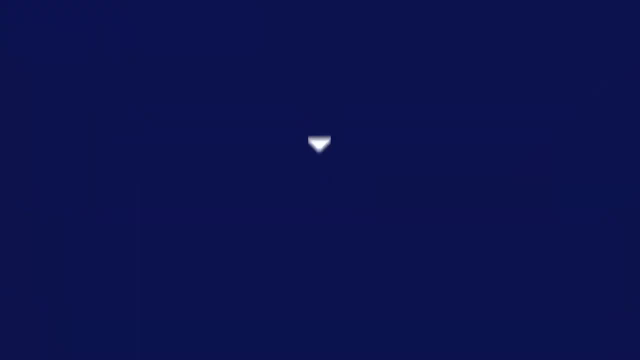 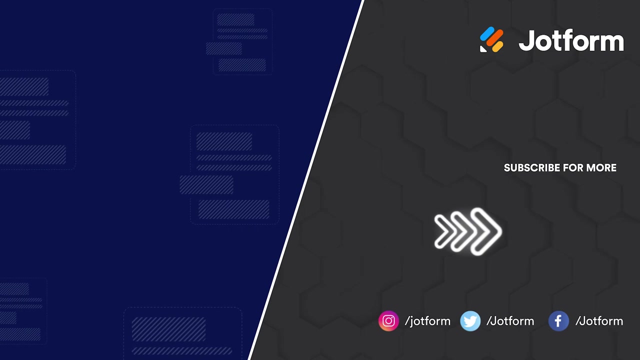 Cross-tabulation comparisons: Tools for survey analysis. JotForm Report. Builder. Once again, I'm Marquesha and I'll see you all later. JotForm Report. Builder.